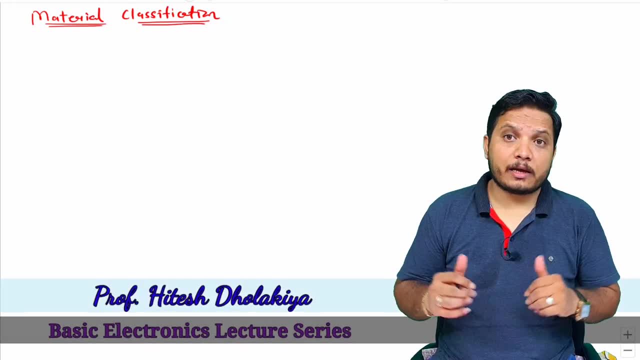 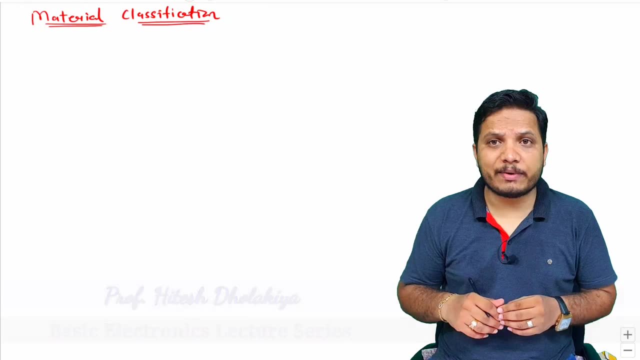 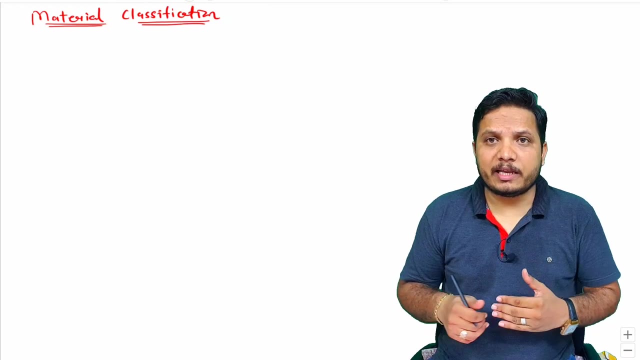 Welcome to basic electronics lecture series. I. professor Hitesh Dholakia is going to explain you material classifications based on its conductivity in this video And at last we will see how energy band diagram is there with different materials based on its conductivity. So when we want to 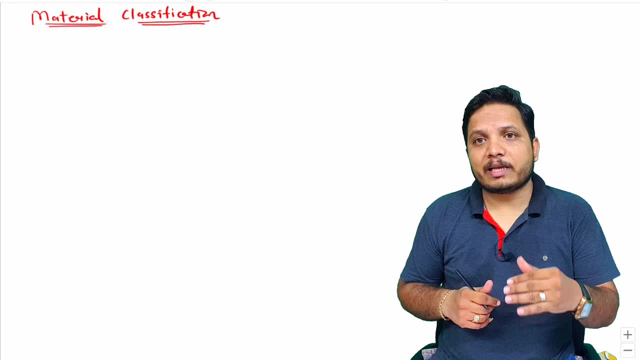 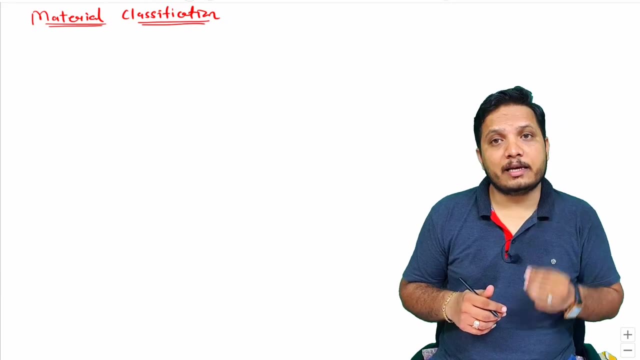 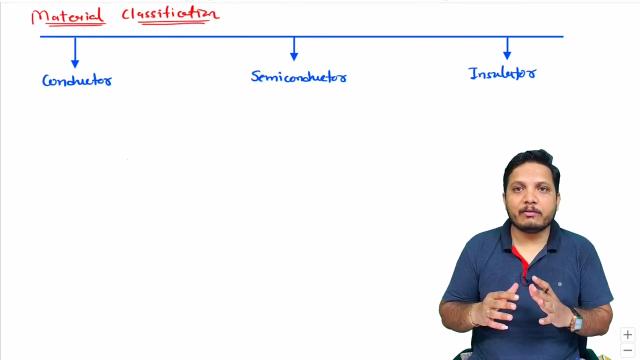 classify material based on its conductivity, then one can classify that in three categories: One is conductor, second is semiconductor and third is insulator. Now let us try to understand this material with respect to its conductivity. Now see, when we talk about conductors, then one can say: with conductor, if you apply. 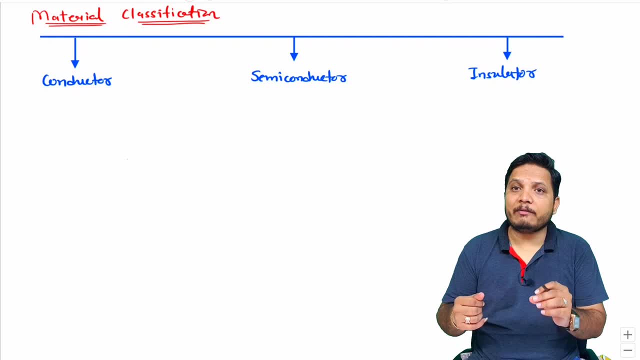 smaller potential across material, then even it will pass current through the conductor. So when we talk about conductors then one can say it will pass current through the material. But in case of semiconductor material at smaller potential across material it does not allow flow of current. but after somewhat higher 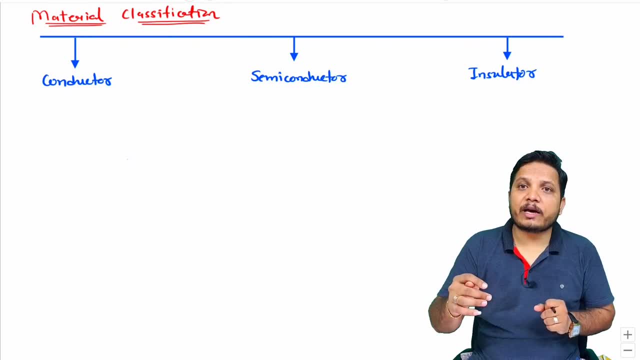 potential. it will allow passing of current through the material And in case of insulating material, you will be observing at very high potential across material. it does not allow flow of current. Now let us try to understand the whole basic slide. Conductivity is very high with conductors, it is moderate with semiconductor and it is 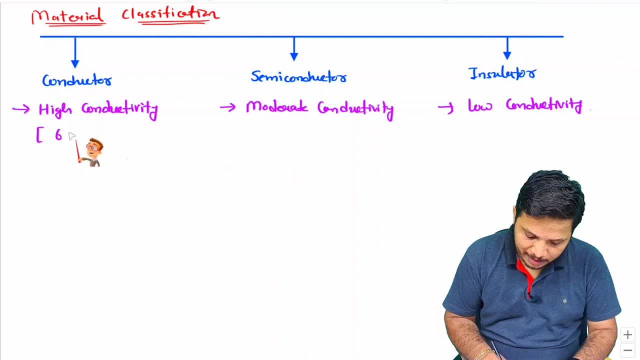 very low with insulator. Now see with conductor, you will be observing conductivity is greater than 10 to the power, 7 per ohm meter. One should know the basic unit of conductivity, that is per ohm meter, ohm meter, and it should be greater than 10 to the power 7.. Semiconductor material is having 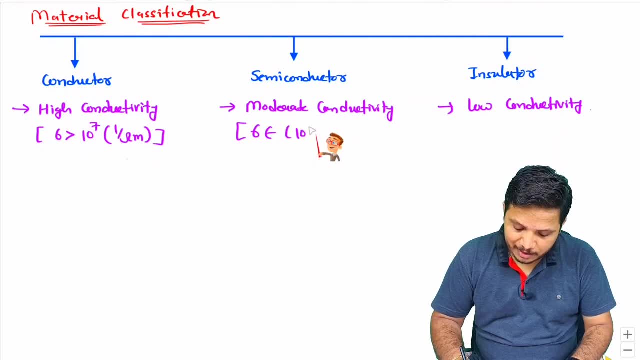 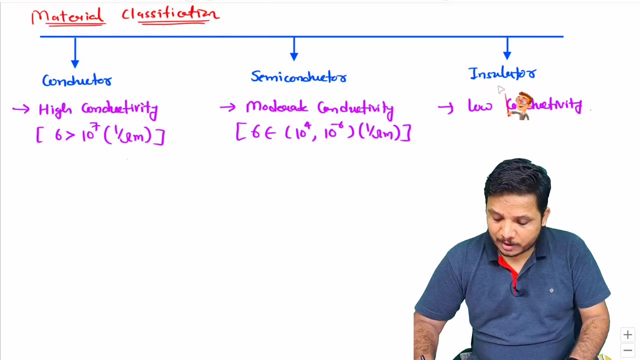 conductivity, which is there in between 10 to the power, 4 to 10 to the power minus 6 per ohm meter, which is referred as moderate conductivity, and in terms of insulating materials conductivity, you will be observing conductivity that is lower than 10 to the power minus 10 per ohm meter. 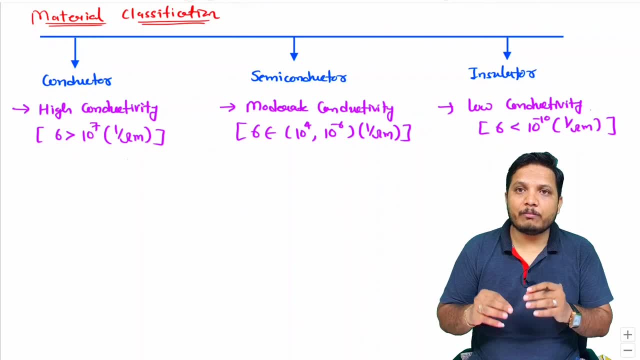 So here conductivity is very low means it should be lower than 10 to the power, minus 10 in case of insulating material. Now one should know: see, conductivity is equals to 1 by resistivity means resistivity is reciprocal to conductivity. So obviously one can say: 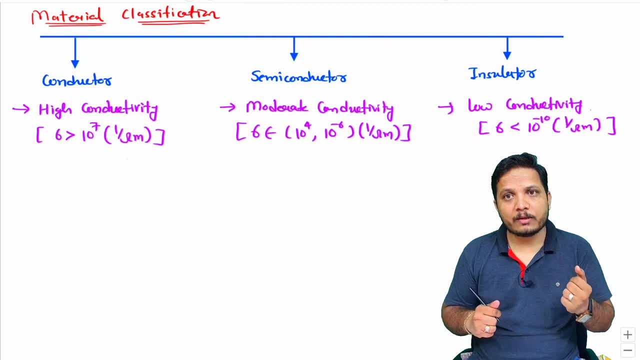 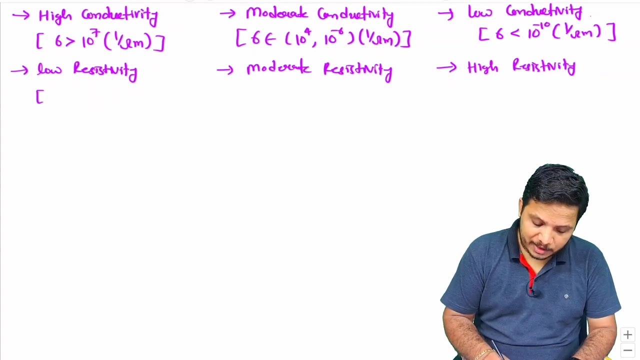 with conductor resistivity will be very low, with semiconductor resistivity will be moderate and with insulator resistivity will be very high. Now, when we talk about low resistivity with conductor, that symbol is rho in most of the books and you will be observing it is reciprocal to conductivity means it should be lower by 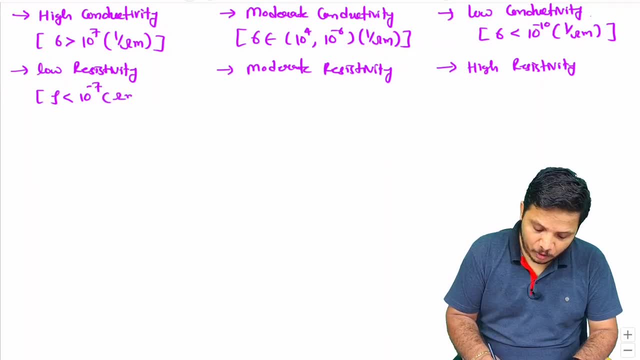 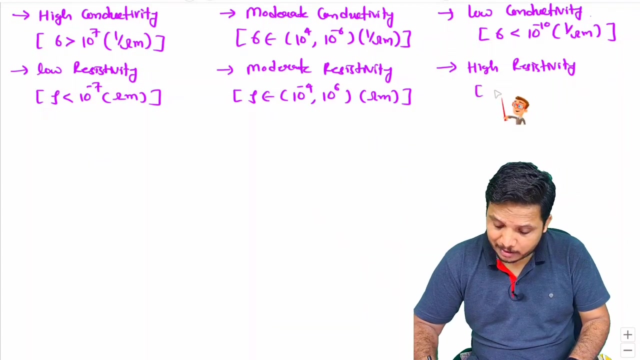 10 to the power minus 7, and unit is ohm meter. and with semiconductor material resistivity, that is there in between 10 to the power minus 4 to 10 to the power 6 in terms of ohm meter, and with insulator resistivity, rho, that will be greater than 10 to the power 10. 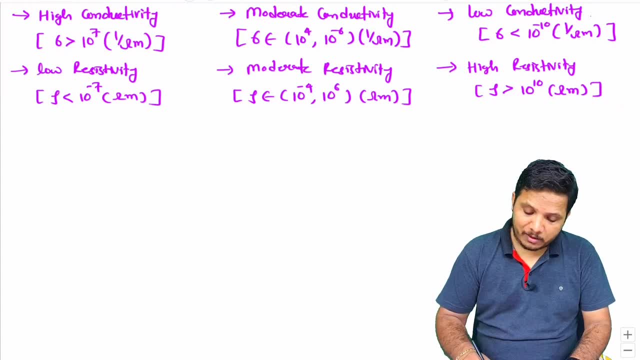 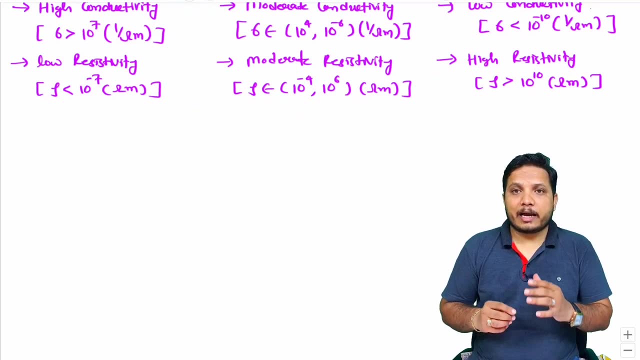 ohm meter. So this is how resistivity and conductivity that is there with this three different materials, and one should know some basic examples of each of these three materials. see with conductor. one can say basic examples are like copper and aluminium with semiconductor widely used. 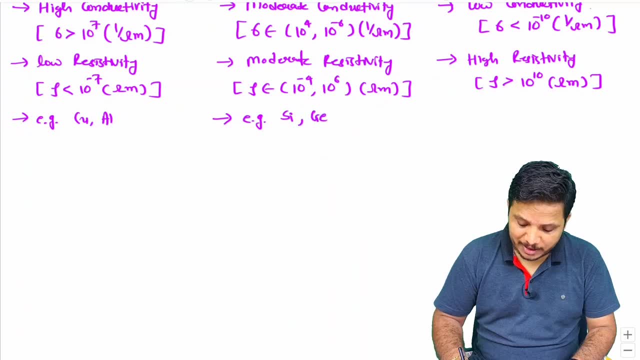 semiconductors are silicon and germanium And with insulator, basic examples are like wood, mica or one can say rubber. So there are many different insulating materials right now. before I explain you energy band diagram of each of this material, first of all one should know the basic structure of 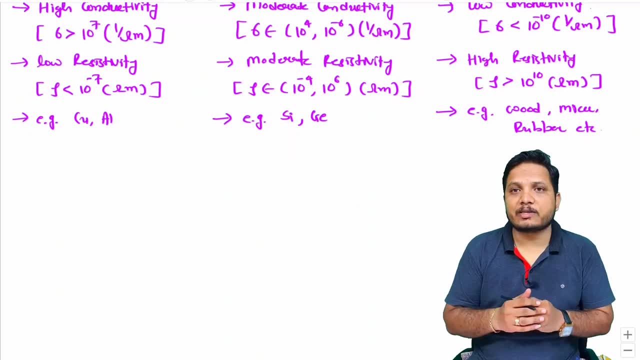 atom And after explaining you basic structure of atom, And after explaining you basic structure of atom Step by step, I will explain you how energy band diagram is there with this: three different materials. So here, when we talk about atom, in center there is proton and neutron. proton is having positive charge. neutron is neutral with charge. so one can say nucleus that is positively charged. Now around nucleus there will be orbits in which electrons will be there. Now around nucleus there will be orbits in which electrons will be there. Now around nucleus there will be orbits in which electrons will be there. 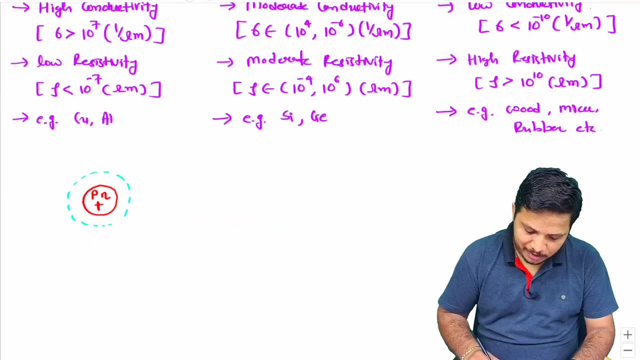 They can be love, the same molecules in that nuclear element. Now I'll give you the diagram. in first orbit, you will be observing, there are two electrons. So you see, in first orbit there are two electrons. right in second orbit there are 8 electrons. 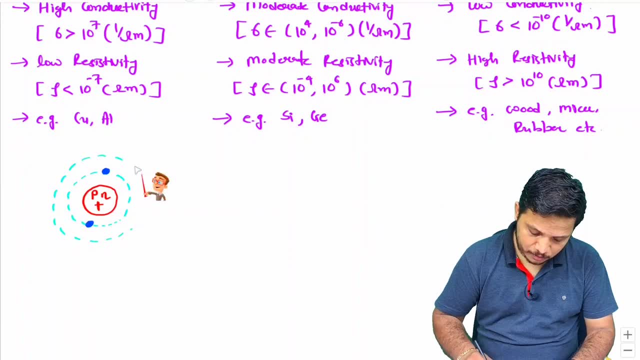 Here they have two electrons in first orbit. New segundo órbital tiene cinco electrones. Let me draw one more Orbit. you will be observing, you see, aам psí, second inbox, a accustomed atmosphere and galaxy will increase. but here I'm not going to draw many electrons without the orbit. Here there is an emba pardon sign of weakness, like magnifying the energy band diagram. This means that when you are considering pulsing a purpose, it has some ê libre, and this is to do with the energy injected into the pole and the energy on the pole. 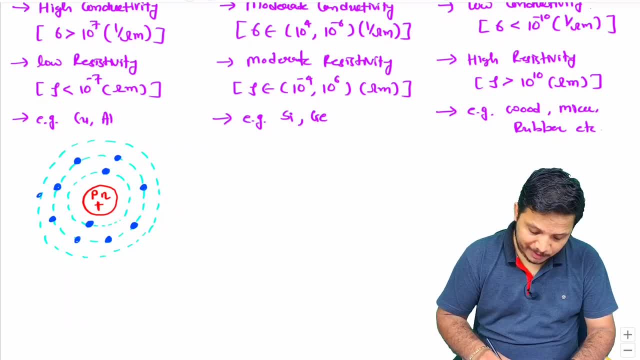 This also means that lot of free electrons present in the- eventually the previous- galaxies are asked to be shifted to reason antenna. Let us say there are few electrons which is there with outer orbit. So I am drawing three electrons with outer orbit, Right. 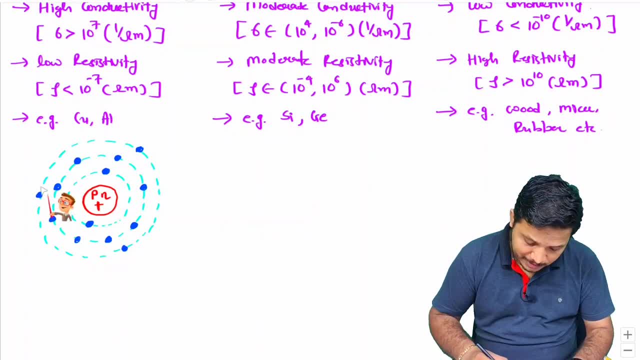 Now, here there are few basic things that one should know. See, this is the most outer orbit that is having few electrons. Here, in this case there are three electrons, So energy band associated with these three electrons is there in valence band. 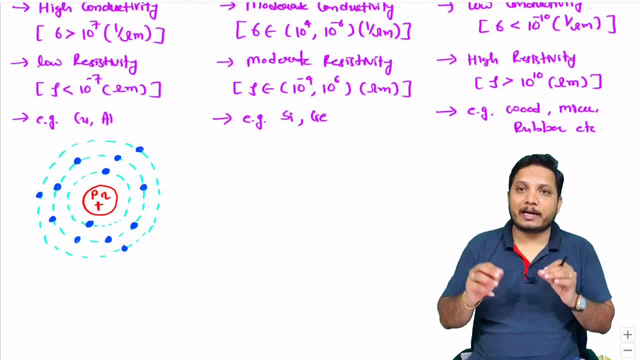 Right. So when electrons are there in orbits, at that time energy associated with those electrons is there in valence band And if you want to flow current, in that case those electrons should jump from valence band to conduction band. 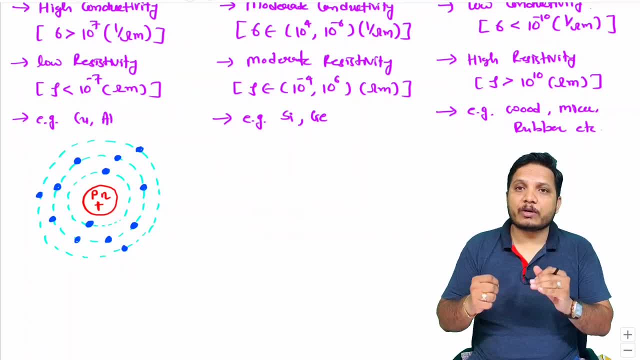 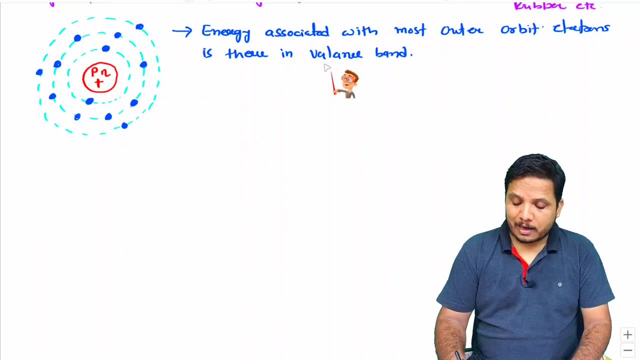 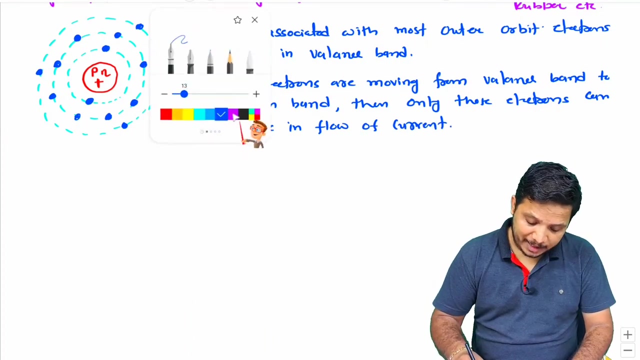 Then only there will be flow of current because of those electrons. When electrons are moving in conduction band from valence band, then only there will be flow of current. Now let us try to understand all those things by energy band diagram. 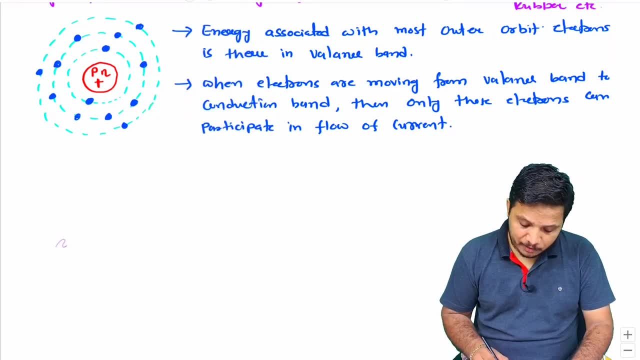 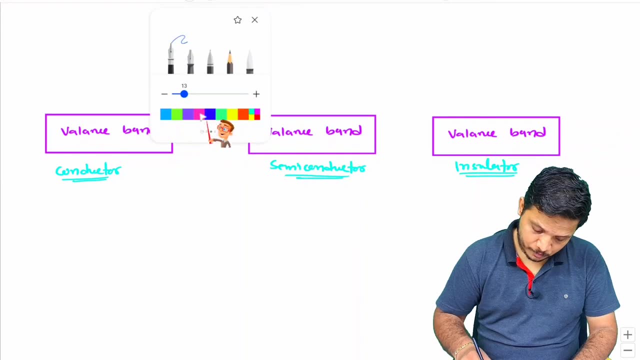 So first I am drawing valence band for all three materials. Now, when we talk about conductor, at that time you will be observing valence band and conductor. So what happens is valence band and conduction band is overlapped to each other. 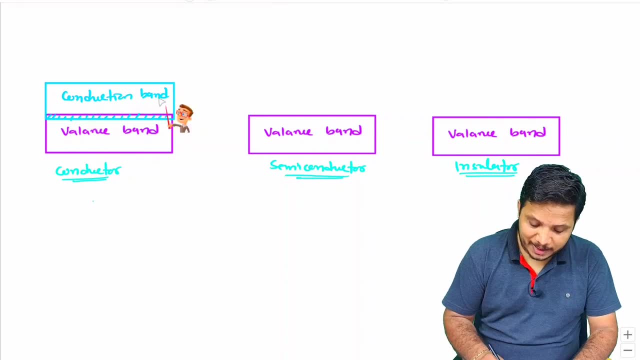 Let me show you that. So you see, here valence band and conduction band is overlapped to each other. So what happens is electrons which are there in valence band does not need energy to jump inside conduction band, right? 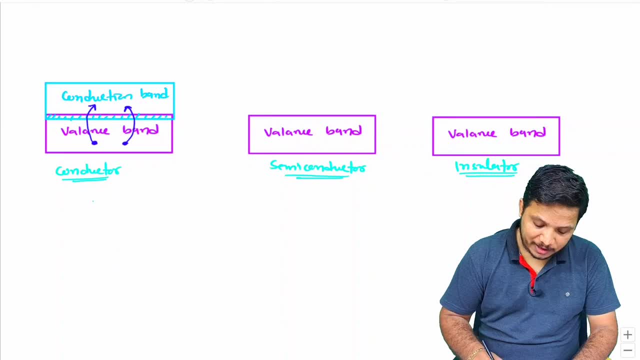 As conduction band and valence band are overlapped to each other At lower potential across material, there will be flow of current. But when we talk about semiconductor material you see there is a gap in between valence band and conduction band. 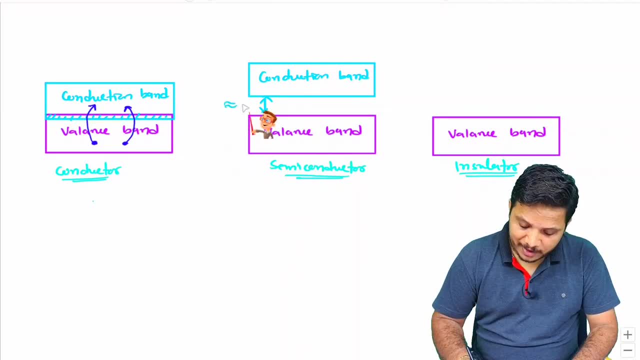 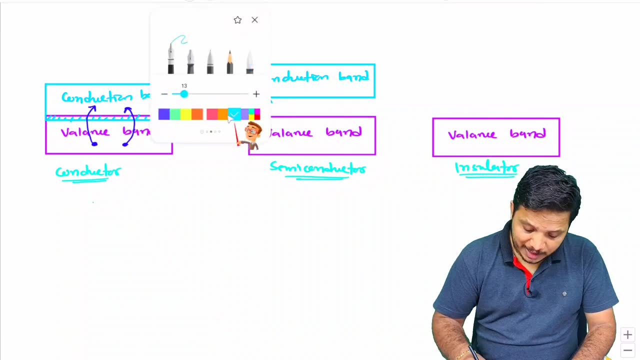 and this gap that is there somewhere nearer to one electron volt, right? So what happens is electrons which are there in valence band. it needs one electron volt energy to jump in conduction band. after that only there will be flow of. 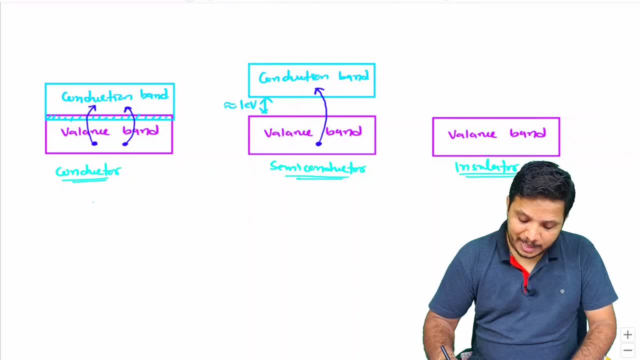 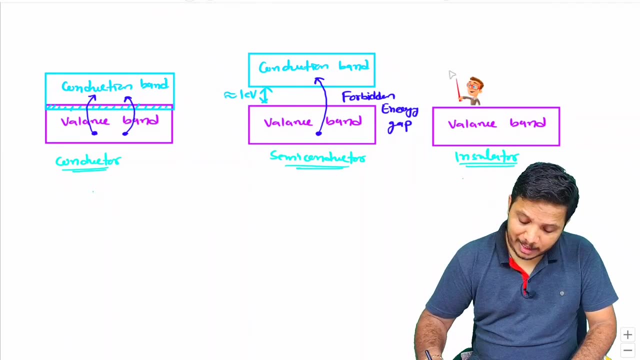 current right and this energy gap that is referred as forbidden energy gap. Now, when we talk about insulating material, then you see conduction band and valence band are separated by energy band gap that is very high and this energy band gap that is greater than 6 electron volt right. 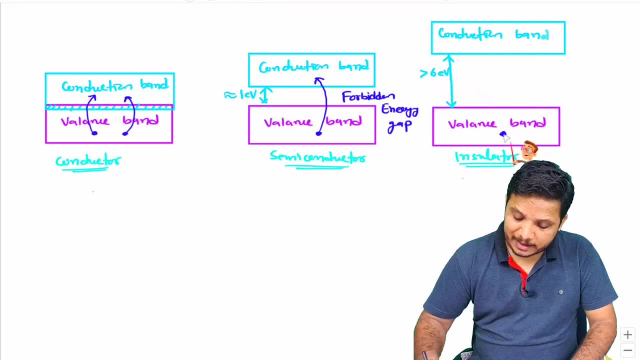 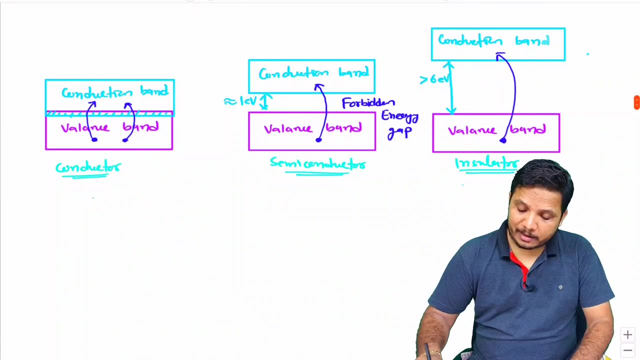 So what happens is if you apply greater than 6 electron volt energy to electrons, then only it will move into conduction band and it can participate in flow of current. So this is extremely, very high energy which is required to give to electron. So one can say, in electron at very high potential even one cannot flow current. 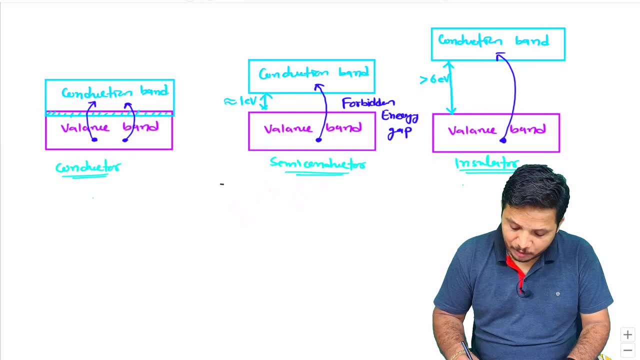 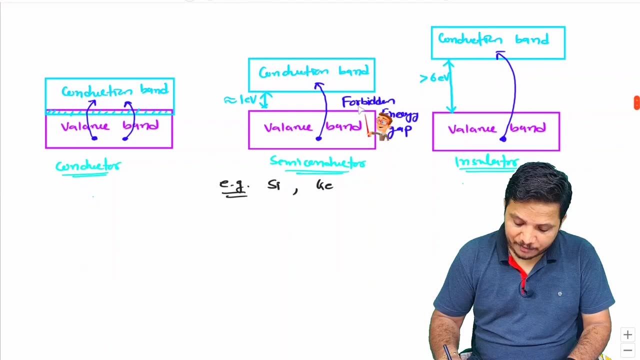 Now you see, here in semiconductor material We have two examples that I have already told you: silicon and germanium. and if you talk about forbidden energy gap which is there with silicon, then that is 1.16 electron volt and with germanium material, you will be observing that is 0.75 electron volt. 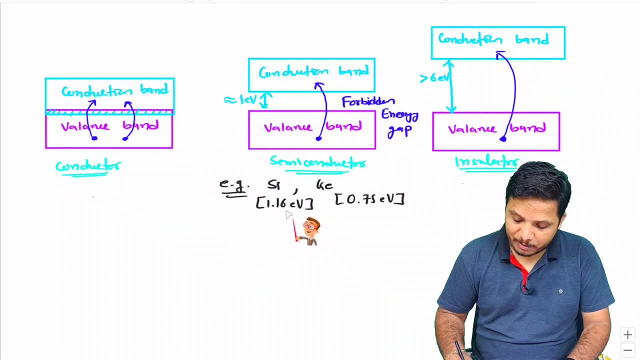 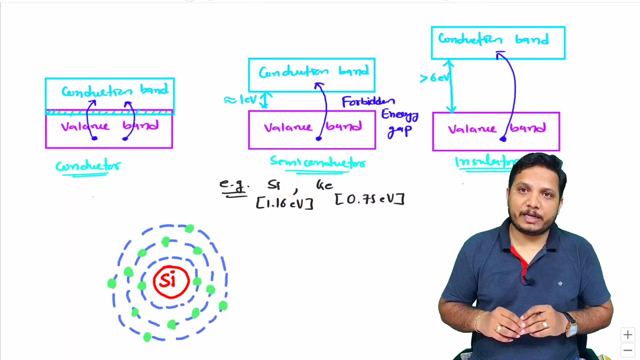 So why silicon is having higher forbidden energy gap compared to germanium. So that is what one can observe by its atomic structure. You will be observing, silicon is having lower number of orbits right, And germanium is having higher number of orbits.